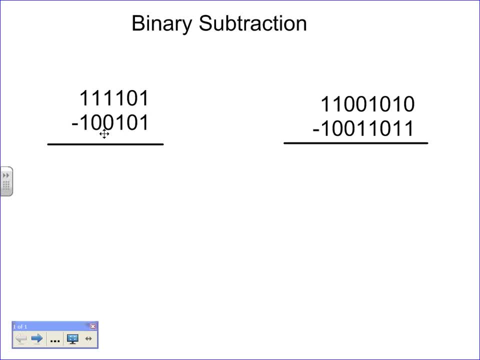 to borrow from the column to the left. So if we take a look at this first example, I know just by looking at it that the number above that I'm subtracting from is larger than the number I'm subtracting And I can easily go through this number, no problem. So I have 1 in the first. 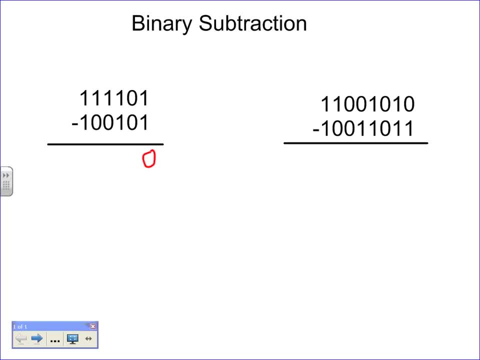 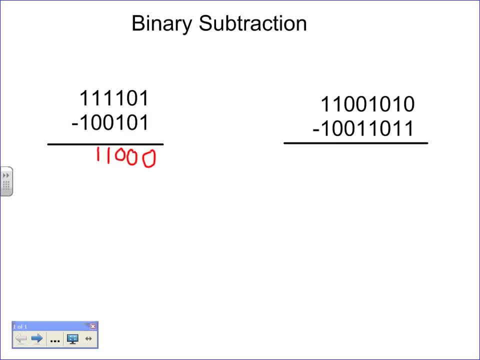 1 minus 0 is 1.. 1 minus 0 is 1. And 1 minus 1 is 0. And we don't have to put that first 0, because it's the leading 0. And there's our answer, And that should be no surprise, and that one's pretty. 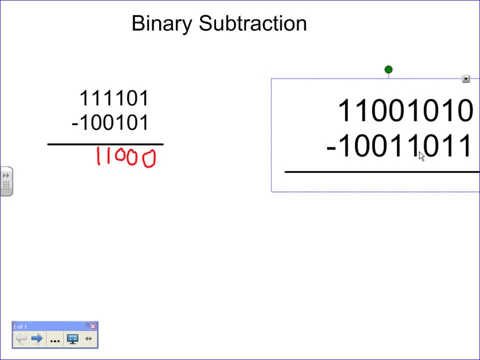 simple. If we take a look at our second example here, this one's going to be a little bit tricky because we're going to have to borrow, And borrowing is not too bad. It's similar to, like I said, to, normal decimal subtraction. So the first character. 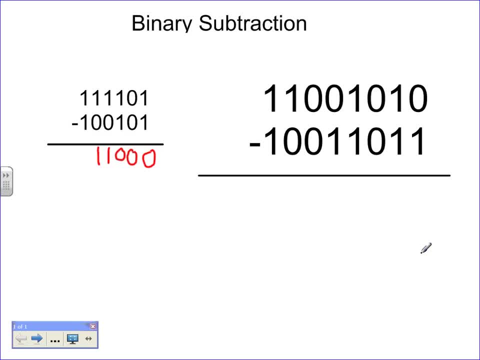 first side we subtract is the rightmost side, always just like regular subtraction. So I have 0 minus 1. And for this I have to borrow. So for me to borrow, I have to cross this one out and make it a 0, okay, But when I bring over that 1 into the column to the right of it, 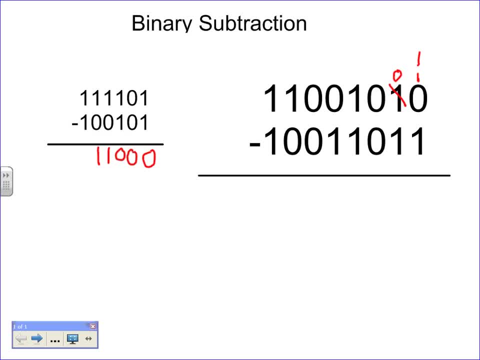 it becomes two 1s. So it's just the opposite of what you did when you were adding. So now I have two 1s, one of which will be subtracted, So this one here will be subtracted from this one here. 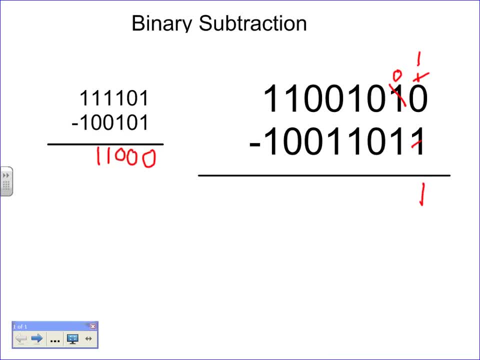 And we subtract this one here from this one here, And we subtract this one here from this one here- would have a remit. we would have a one left over. our next step: we do a zero minus one again, and this time again we'll have to borrow. we can't borrow from the columns to the left, so we're. 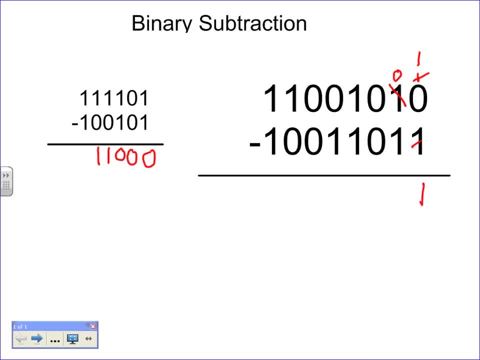 going to have to go two columns over, so we're going to borrow from this one. it becomes a zero and this one would get two ones, one of which we're going to borrow. so this one's gone and we have two ones and we can say that that means that we have, we can subtract from, maybe, this one. 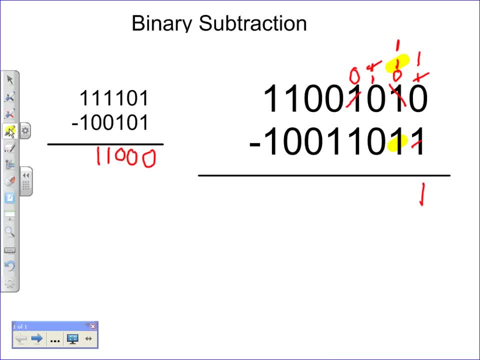 and this one, leaving again just that single one in the next column. i now have one minus zero. that's one. this one, i have zero minus one and again we're going to have to borrow all the way from the next one. we find that'll leave zero. 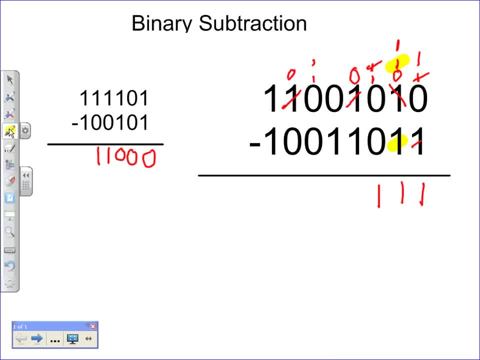 this will leave two ones. we're going to cross one out because we're borrowing it for this one, and we're crossing one out to borrow for this one, so we'll have one minus. so there's two ones, one and one minus the one down here in our original, so we'll be left with the remainder. 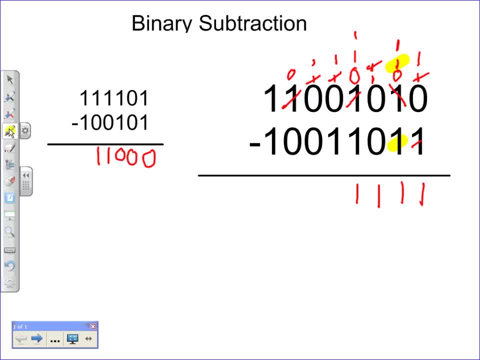 of one down there and the next column we have: we have the one minus the one, so we have a zero. then we have a one minus zero, so we have a one. a zero minus zero is zero, one minus one is zero. so we don't even really need those two zeros. and there's our answer. 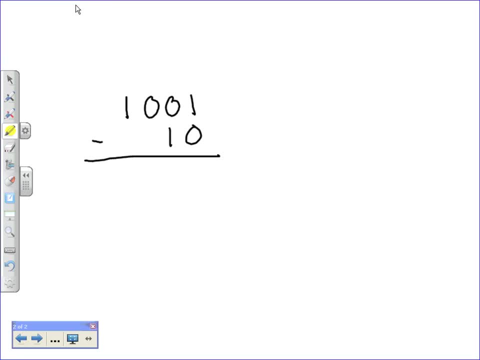 so let's do another example, and a simpler one, just so we can make sure that what we're doing makes sense. so if we have starting at the right one minus zero, we know that that's one, and again we go to the next column: zero minus one. we're going to have to borrow from here. 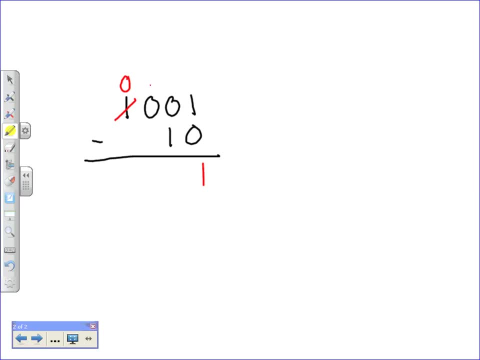 so we make that a zero, it becomes two ones. in the next column we're going to have to borrow one of those, and it becomes two ones in the next column. so two ones minus one of those leaves us with one. the next column is one minus zero, leaves us with one, and we're done. 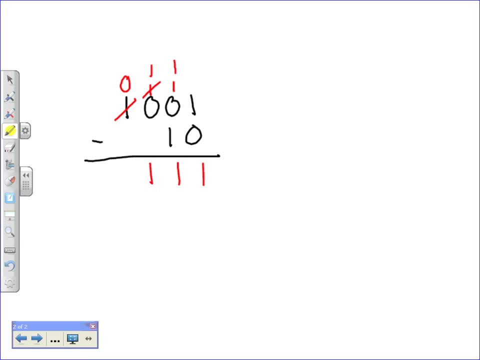 and we can check this. so we know that one zero, zero one, in decimal form, if, since we know that this would be the ones column the twos, column the four and the eight, that one zero, zero one is nine, and we can also check that one zero would be one zero and we can also check that one zero would be.